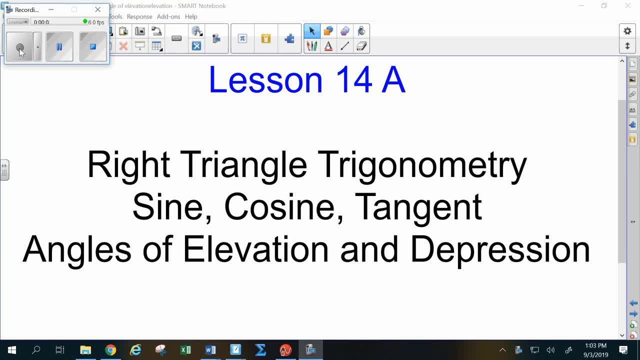 We are reviewing right triangle trig today, part of what is in Lesson 14. We are going to be looking at what sine cosine and tangent mean in right triangles and we will be reviewing angles of elevation and depression. So we will start with some picture vocabulary for angles of elevation and depression. 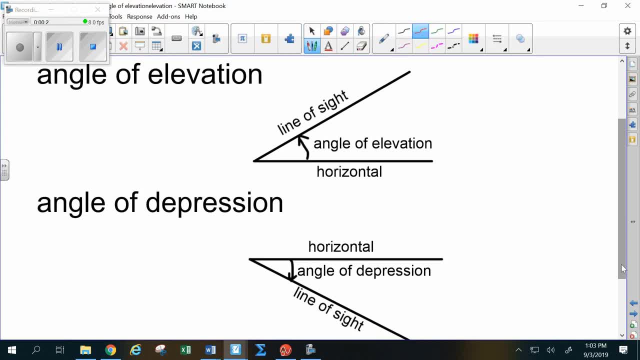 Notice: these never, ever, ever, ever use a vertical line. They are always a horizontal line and a slanted one. If we are talking about an angle of elevation, we are looking up at something else and we're talking about how much do we have to take? 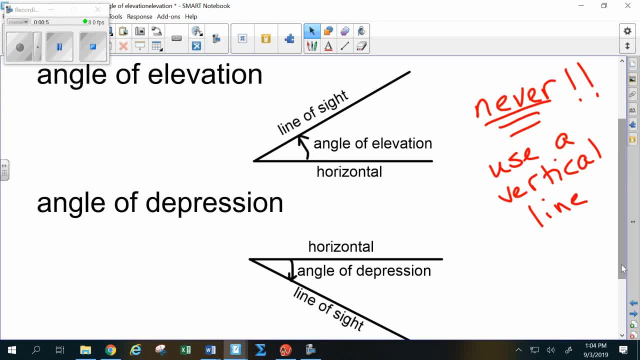 We need to tilt our eyeballs up to take a look at whatever we're looking at. If we are talking about an angle of depression, we are in an airplane, we're at the top of a cliff or the top of a building. we are looking down. 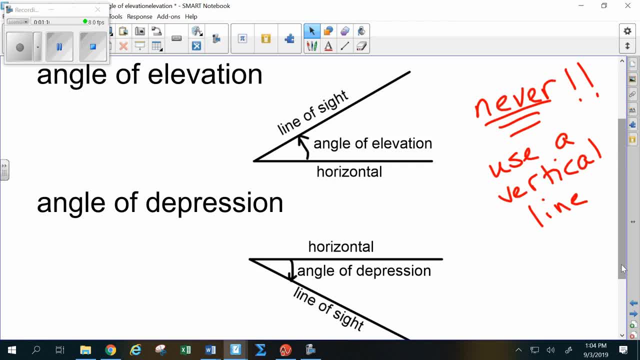 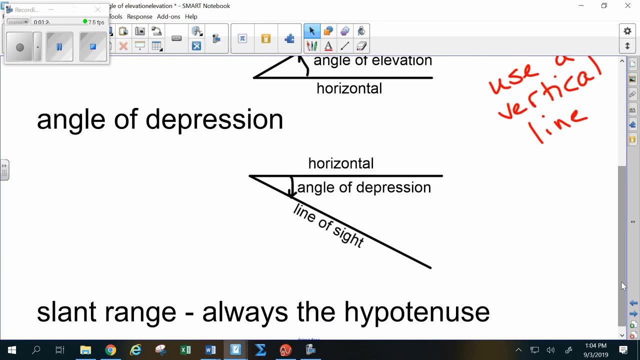 we're talking about. how much do we need to tilt our eyeballs down to be able to see whatever the object is that we are sighting? Another vocabulary word that your book sometimes uses is slant range, Which is always that slanted line, the hypotenuse. 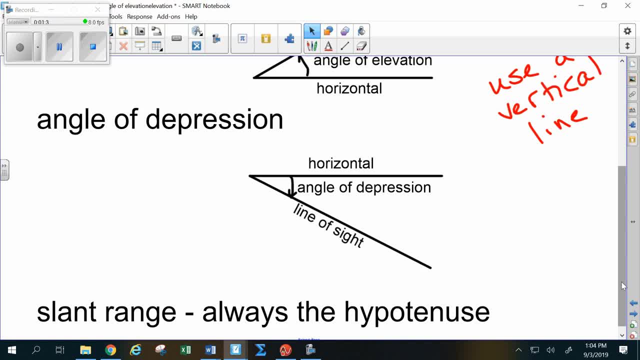 Sometimes the word problems will say the slant range is or what is the slant range, and I just want you to know what they're talking about when you see that vocabulary item On the next slide we will fill in our formula list with that way we have of remembering sine. 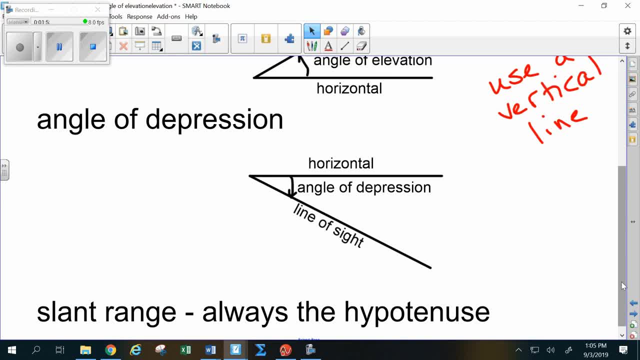 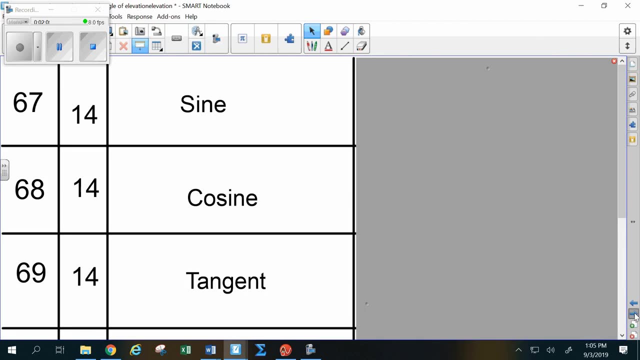 cosine and tangent For a right triangle. Does anybody remember the little funny sounding mnemonic word we use to help us remember Emma, It definitely is SOHCAHTOA, So we are going to start off with that today. So S-O-H-C-A-H-T-O-A. 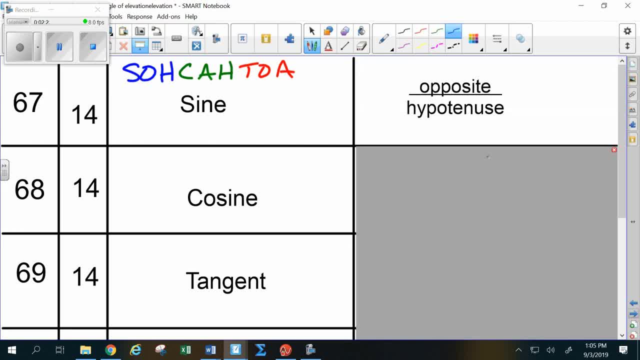 Which simply means if we have a right triangle, it's only for right triangles. If we are talking about the sine, the O and the H mean opposite over hypotenuse. If we are talking about cosine, A-H means cosine will be adjacent over hypotenuse. 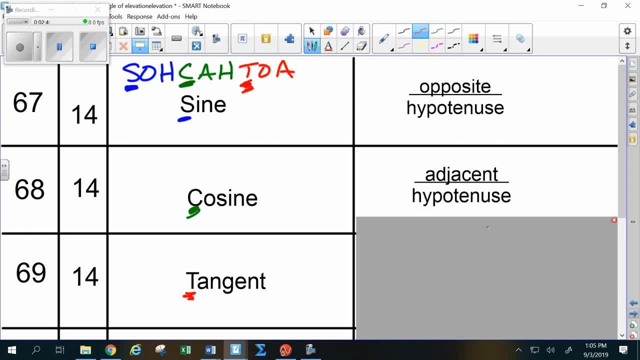 And if we are talking about tangent, O-A means that ratio will be opposite over adjacent. We only have a hypotenuse in a right triangle, so ratios set up this way only work in right triangles. Later this semester we will be working with other kinds of triangles and using trig on those triangles as well. 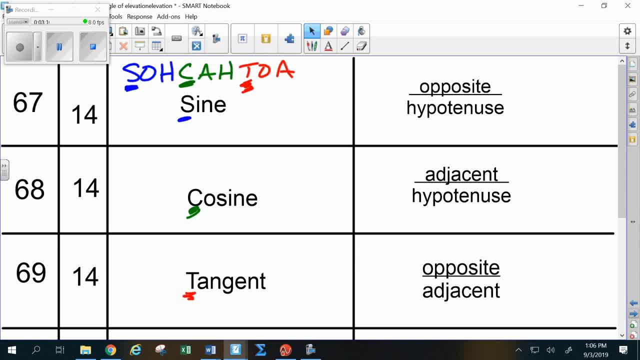 But for right now we are only reviewing right triangles. You only have a hypotenuse in a right triangle, So SOHCAHTOA does not work if it is not in a right triangle. It only works if the right side of the triangle is set up in the right triangle. 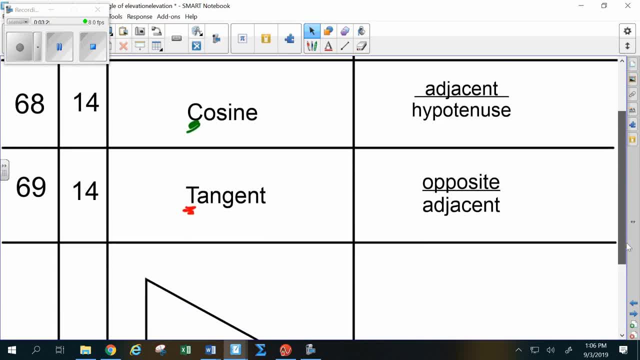 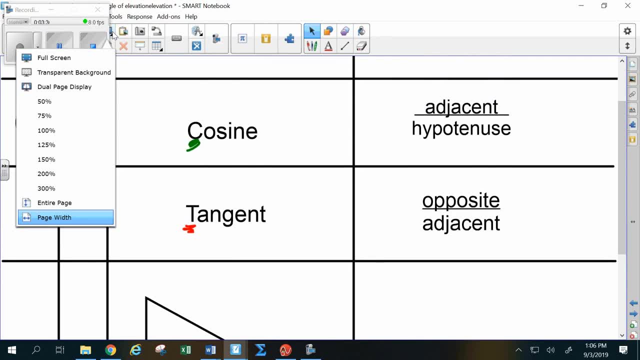 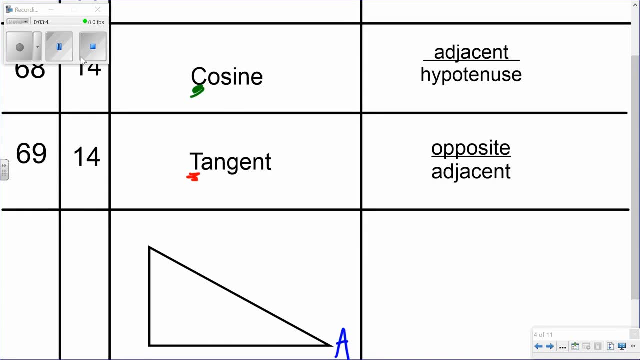 So if we are talking about a right triangle, we have something like this: So if this is my triangle and maybe I call this angle A and this angle B and this angle C, So then I will use lower case for the sides. 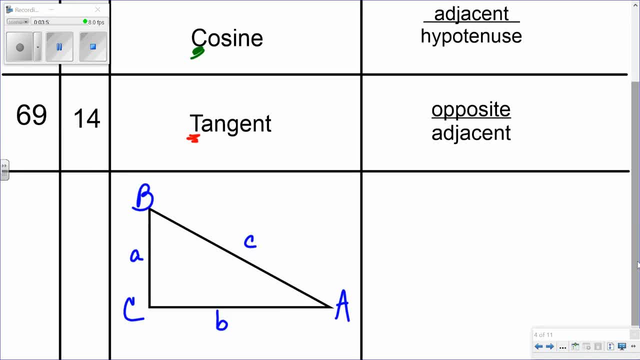 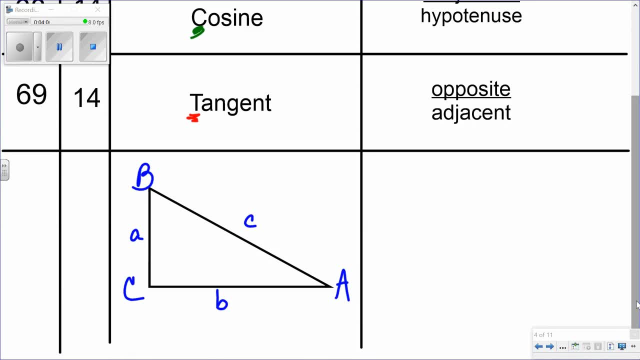 that is standard math notation. Lower case for the right triangle for sides, uppercase for angles: big A and little A are across from each other. So if I want to talk about angle A to begin with, for angle A side A is opposite, side B is: 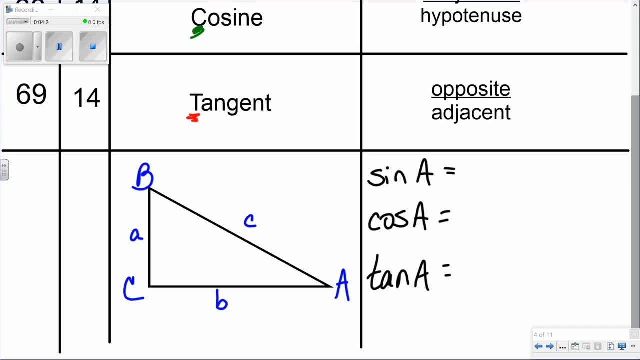 adjacent, C is the hypotenuse. So for angle A, opposite over hypotenuse is A over C. For angle A, B is adjacent, So adjacent over hypotenuse is B over C And tangent is opposite over adjacent. So for angle A, opposite would be A, adjacent would be B and we have A over 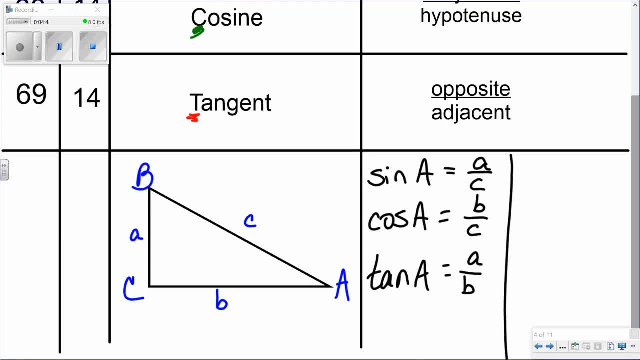 B. If, however, I switch to the other angle, watch what happens If I take, I'm going to write B there. if I take the sine of angle B, for angle B, the opposite side is little B and the hypotenuse is still C. So if I want the sine of little B, I get B over C. 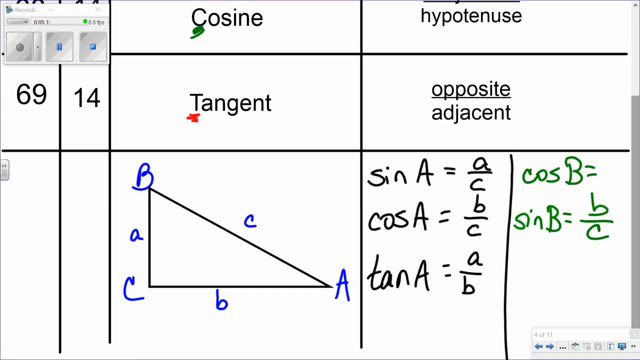 And if I take the sine of little B, I get B over C. And if I take the sine of little B, I get B over C. If I take the cosine of angle B, I'm looking at adjacent A over hypotenuse C, so I get. 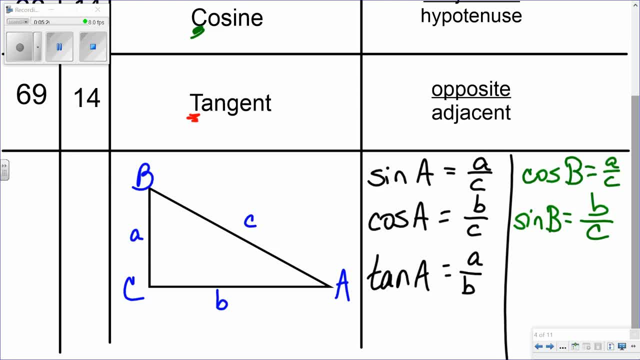 A over C. So in one triangle the sine of one of the acute angles is the cosine of the other, one: A over C and A over C. The other way around, the cosine of one is the sine of the other, B over C in this case. Now, if I do tangent of angle B, I get B over C. 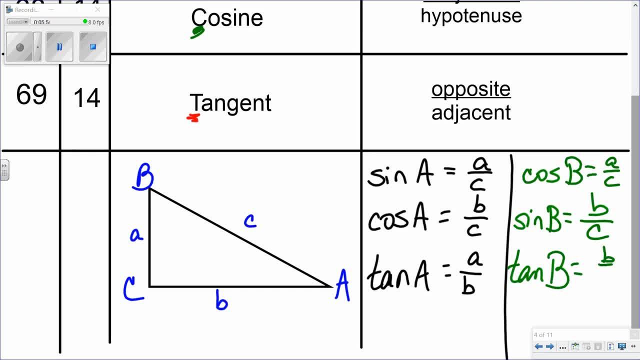 Opposite over adjacent is now B over A, So those are reciprocals. So in one triangle, the two acute angles, their tangents, are reciprocals of each other. Any questions? so far with that? Okay, then let's see what happens if we start to try to use that a little bit. So we have 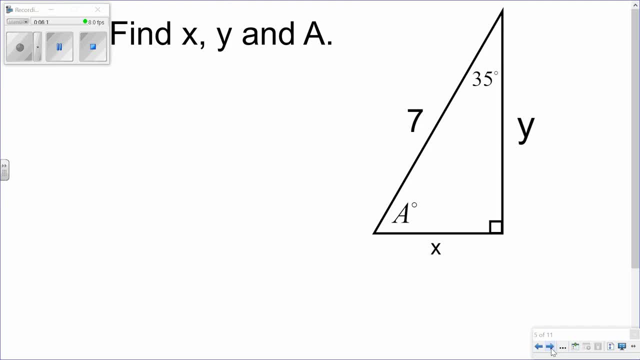 a right triangle And they tell us a 35 degree angle and they tell us one side is 7, and we need to find both of the other sides and we need to find the other angle. So they tell us one side and one angle. Is that right? Do they only tell us one angle? They tell us two angles. 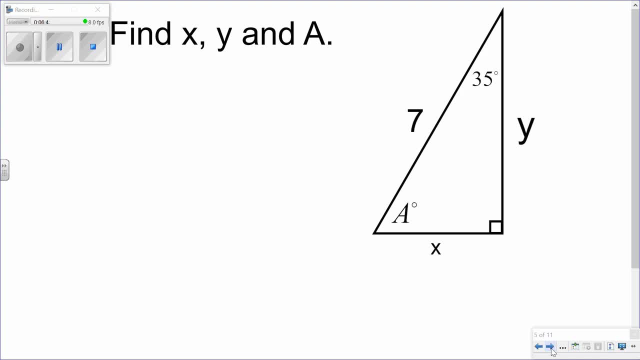 because we also have the 90 degree angle. So how can we find the third angle if we know two triangles, Matthew, Triangle sum. So help me out, Help me do that. That is true. And so then we subtract and get that A is how much, And then I'll teach. 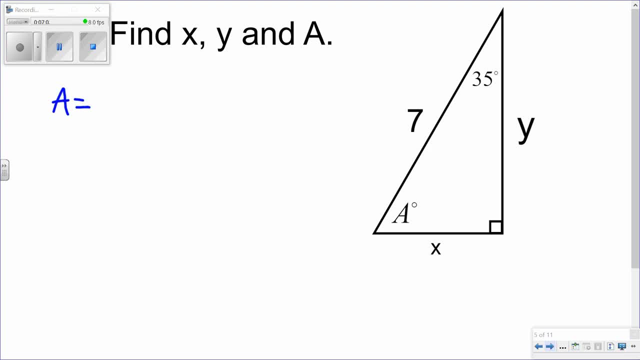 you the shortcut way. So 90 plus 35 is 125.. 180 minus 125 is 55 degrees. It has the degree sign in there. Okay, shortcut. If it is a right triangle, The shortcut only works on right triangles. What do the other two angles have to add up? 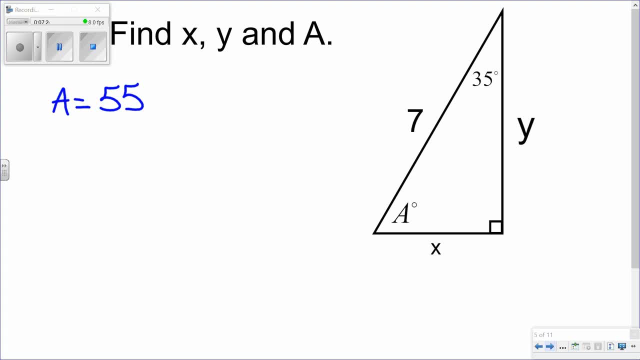 to. So all you need to do is 90 minus 35 is 55. You don't have to do: 90 plus 135 is 125.. 180 minus 125.. Just 90 minus 35. Make it a lot shorter. So now we know this angle And I'm 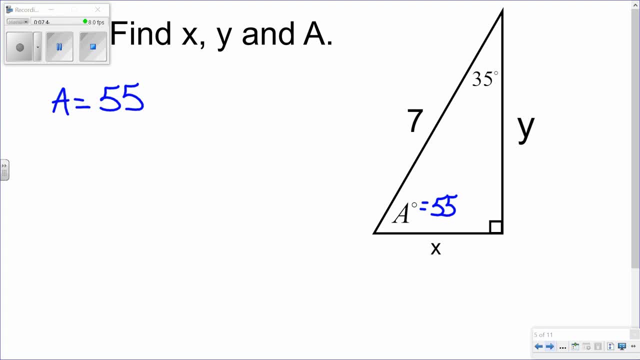 pretty confident that I did it correctly, but I'm only going to use that 55 if I have to. but if I subtract it wrong, It's better to use the seven and the 35 and only use the 55 if I have to. So let's try to find what x is going to be. and can we do that using? 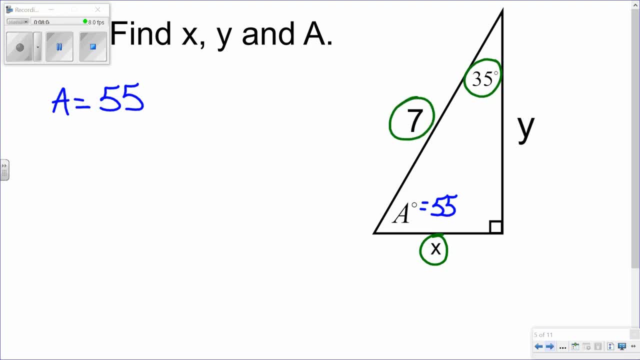 the 35 degree angle and the seven For 35, x is adjacent, opposite hypotenuse to every one, Opposite, and seven is Which ratio does opposite and hypotenuse? Okay, again we'll. So we can say that the sine of 35 degrees is opposite x over hypotenuse 7.. 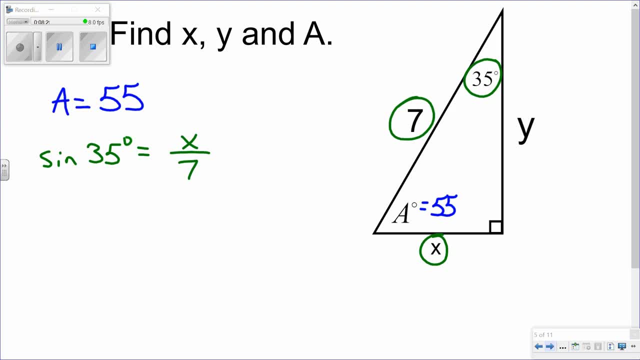 So then how do I get what x is Mia? So x is 7 sine 35 degrees. I want to see that on your papers. Don't go from x over 7 equals to your calculator answer. Write down: this is what you're entering on the calculator. 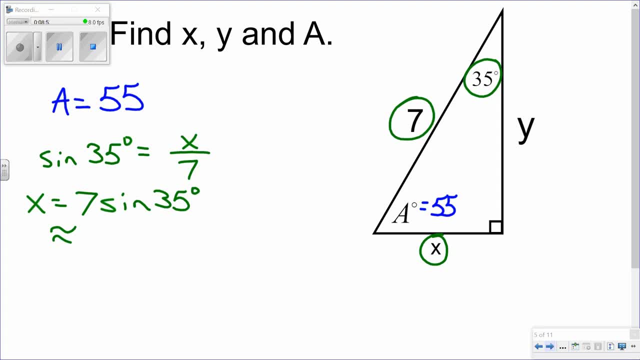 And you don't have to do a times in between there, just 7.. Then here's your trig button on the Inspire. When you push that you get the little chart. Make sure sine is highlighted And then inside the parentheses put the 35.. 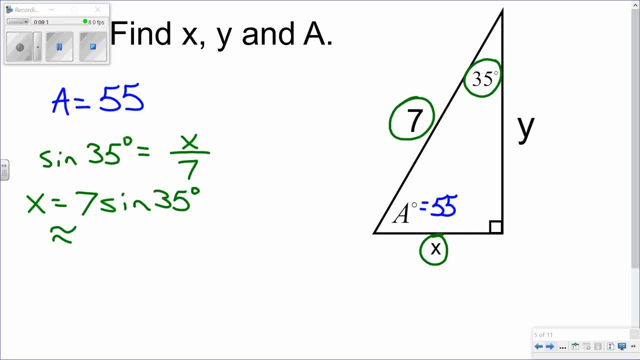 I prefer that you write it this way: Sine 35 degrees And then making sure you go outside the parentheses. times 7 is okay, Definitely not sine 35 times 7, forgetting to go outside the parentheses. That will give you a totally different answer. 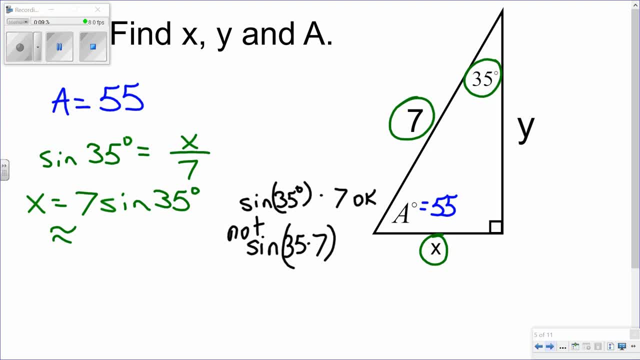 So just trying to review some of the calculator entry tips- And Zoe, you have that. She said 4.015.. Let me see Thumbs up, thumbs down. Is that what others are getting? So we must be in good shape on that one. 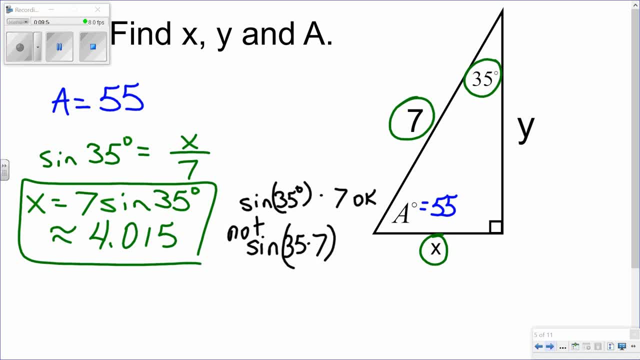 Okay, I could take x squared plus y squared is 7 squared using Pythagorean theorem, But I'd have to store the 4.015.. I can't round it and reuse it, And what if I made a mistake? So it's better to set this one up without using that. 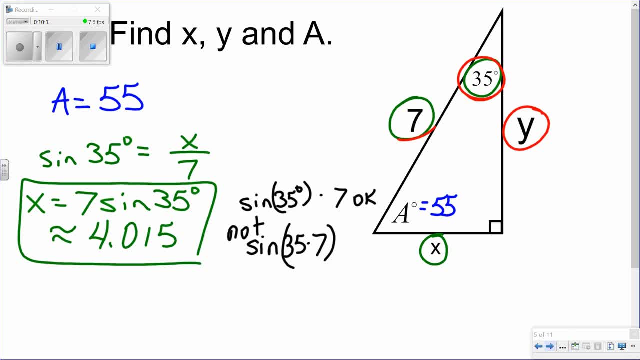 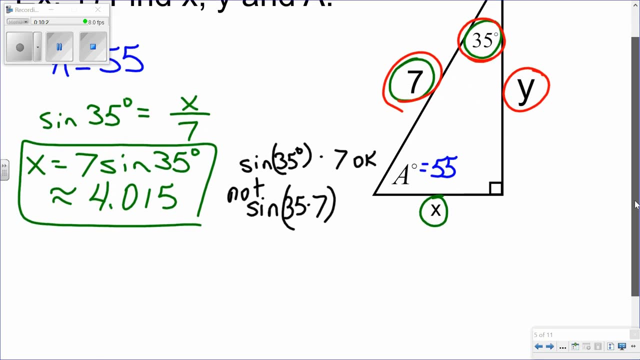 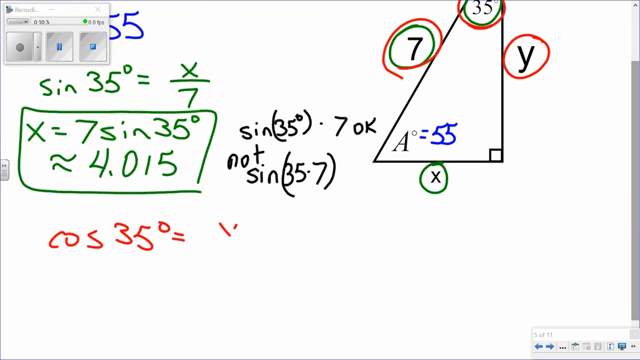 Can we do it using y and the 35 and the 7?? For 35, Blake, y is okay. so adjacent and hypotenuse, everybody is 7.. And adjacent and hypotenuse is which ratio, So we can say cosine of 35 degrees- is adjacent over hypotenuse? 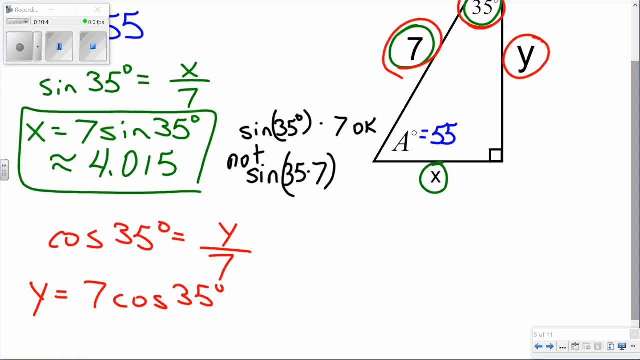 So y is now 7 cosine, 35 degrees, And let me know what you come up with on that one after you have puns Punched it in on your calculators. Lydia, what did you come up with? 5.734.. 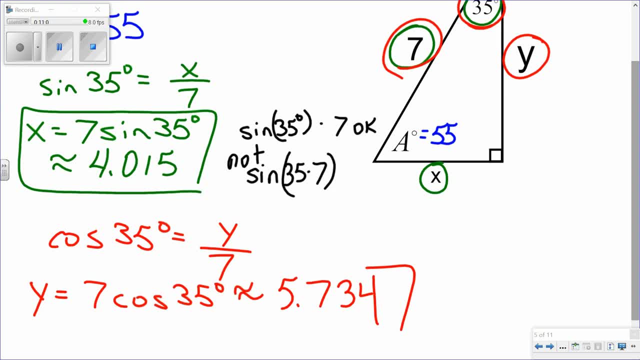 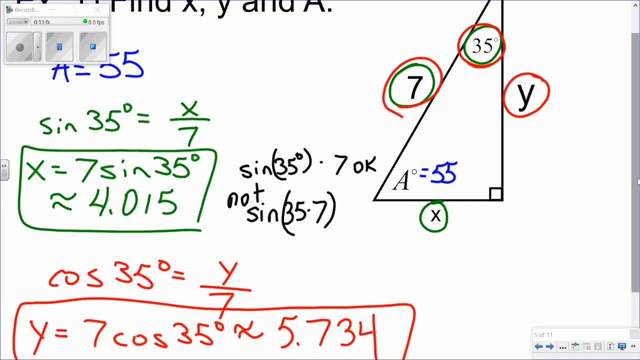 Anybody else getting that? Okay, Looks good to me. also, Anybody with questions on that one. That one was pretty straightforward. Okay Question. This would not have a degree sign because it's a side. So right here, I want you to get in the habit of that, because very soon we're going to start doing things with radian measures. 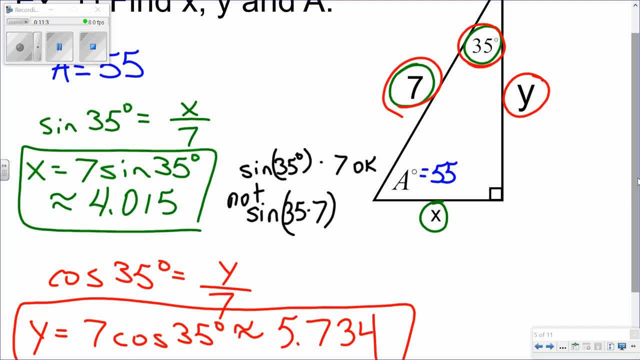 And if it's not labeled, it means radians. And if we didn't have the degree sign, that would mean 35 radians, which is very different from 35 degrees. So we want to get in the habit of if it's not labeled, it means radians. 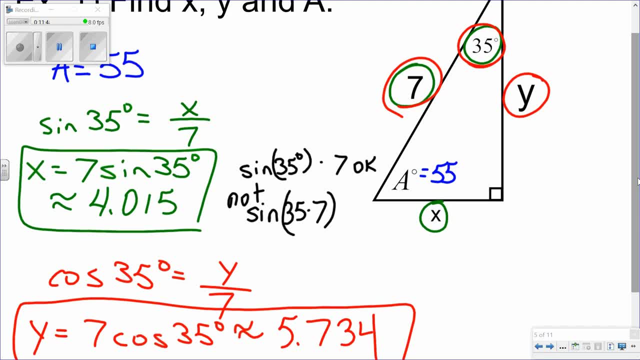 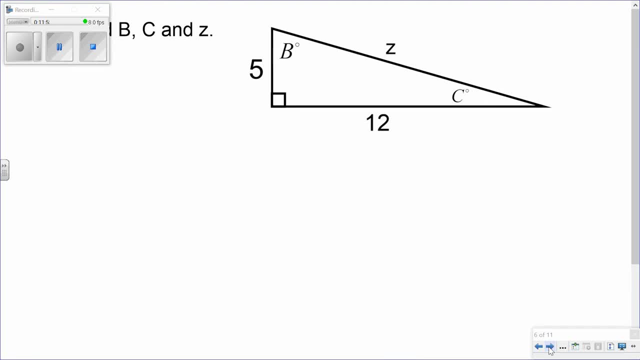 Degrees, putting the degree sign in there. Okay, Next one is a little bit different setup. This time I know two sides and I only know the 90 degree angle. I do not know either of the other two angles, So help me out here. 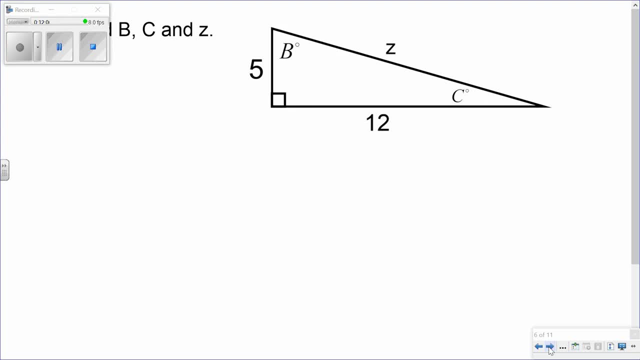 If I know 5 and 12, and I know it's a right triangle, how can I get the third side of a right triangle? What do I need to do for that to happen? two sides of a right triangle, How do I get the third? 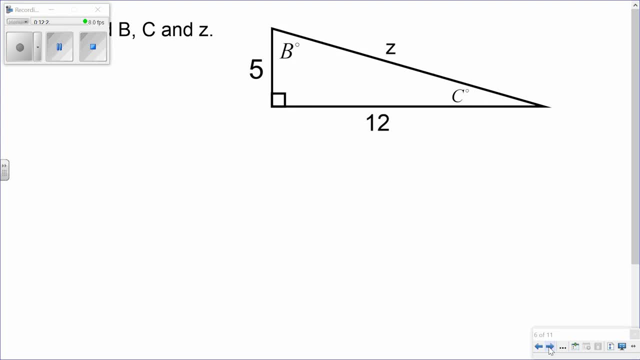 Keith, That's the hard way. What's an easier way when you know two sides of a right triangle and you want the third side? We're going to do the Pythagorean theorem. This one happens to be a triple. Can anybody tell me what z is? 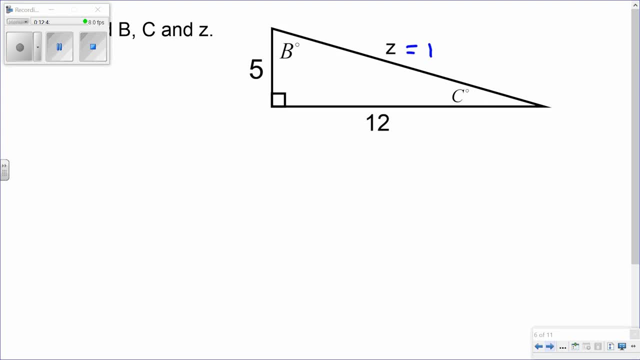 Everybody who knows Thirteen. If you didn't remember, 5, 12, 13 is a triple. You could do 5 squared plus 12. squared, 25 plus 144 is 169, and then take the square root of that. 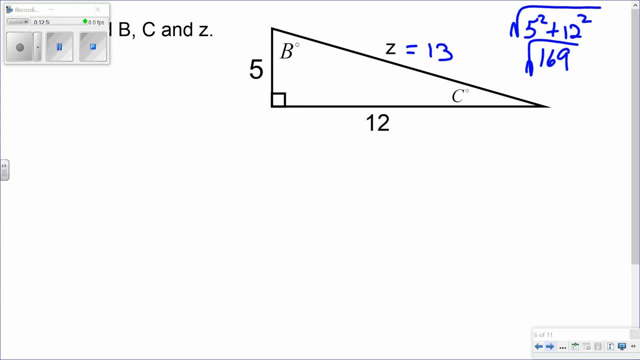 but much faster. if you remember that Question, It's better to just label that as a triple. Now we want to get b and c, So now we're going to be doing what Keith was thinking about. and what were you thinking- b or c- first? 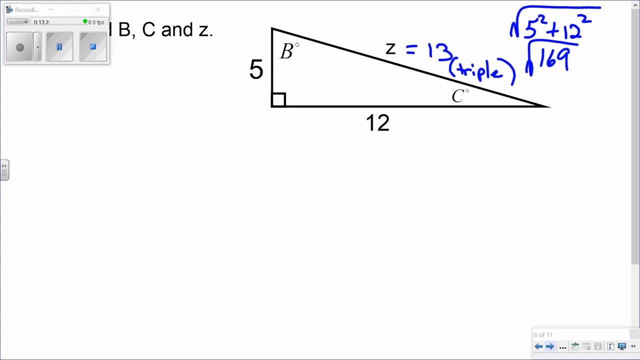 Okay, so if we started with c, what would we write down? What would we write down? So 12 for c is adjacent, opposite or hypotenuse. That's wrong. 10 for c is adjacent opposite or hypotenuse. 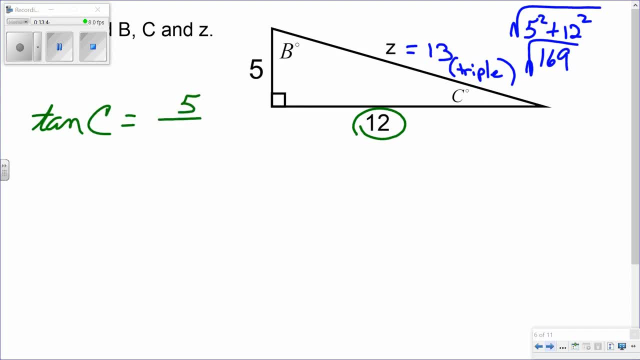 10, for c is adjacent, opposite or hypotenuse, So tangent of c is opposite over adjacent, so 5 over 12.. Is everybody okay with that? Okay, that does not mean c is tangent of 5 over 12.. 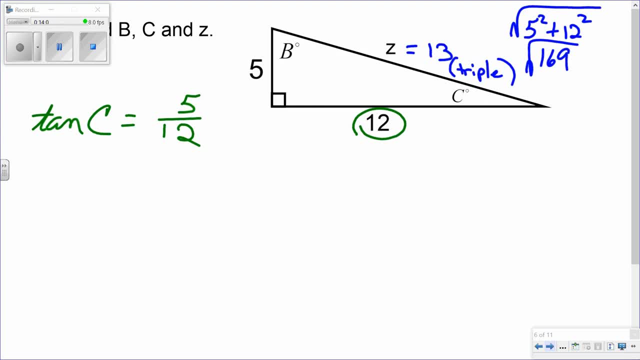 We want to take the angle, the inverse tangent of both sides. This is not tangent to the minus 1.. It's not 1 over tangent, It is the inverse tangent of both sides. So tangent of both sides, tan inverse means the angle whose tangent is 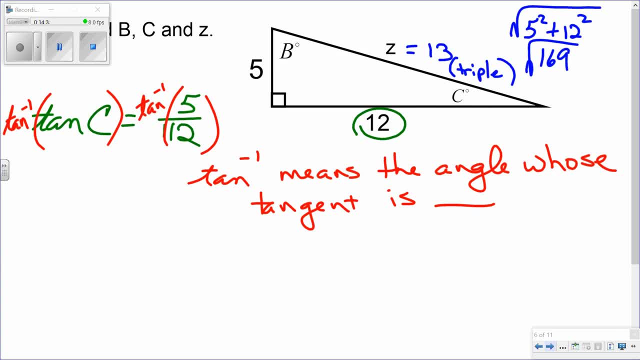 So to enter and then inverse tan of tan cancels out and we just have c is tan inverse. So if we go to our trig button on the inspires in the table, we go to the bottom row, highlight tan inverse. then we put 5 over 12 inside the parentheses. 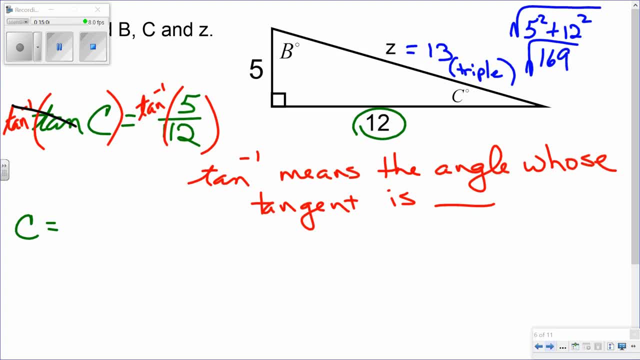 and raise your hand when you know what that would be equal to. Ryan, you have it, Anybody else? 22.620?? Okay, now we know two of the angles. We could do 90 minus the stored value to get the other acute angle. 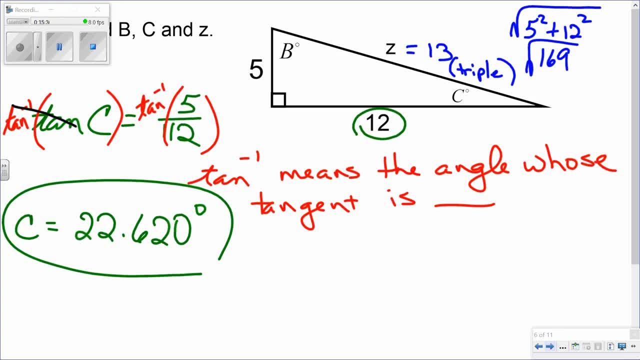 but maybe we made a mistake in there. So it's better to do it without using an answer we found, unless we have to. So we will do. for b, we will say that the tangent of b is its opposite over adjacent, 12 over 5, so we're looking at the reciprocal. 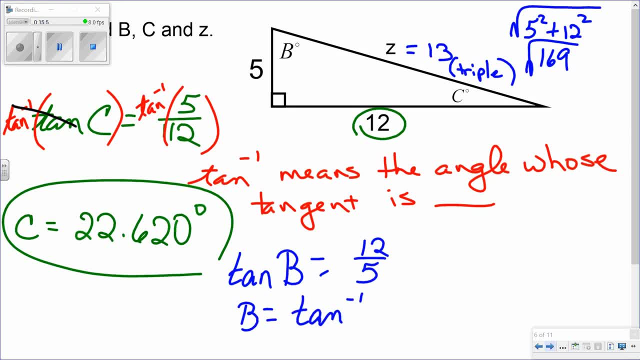 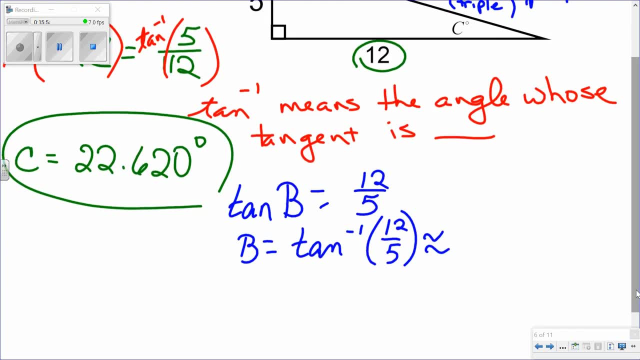 So b is the inverse tan of 12 over 5.. Please enter that on your calculators. Who has that one? Who hasn't already been answering? Some of the others of you have that punched in. who haven't been answering everything already. 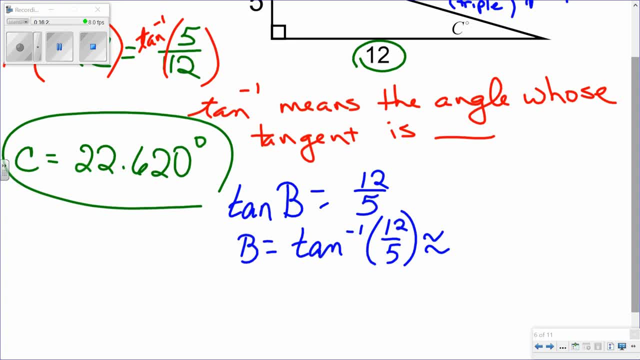 Emily 67.380.. And then, as a nice little check, does it look like b and c add up to 90 degrees? So we don't think we made any mistakes anywhere along the way. Anybody with questions on that? All right, let's summarize the tools. 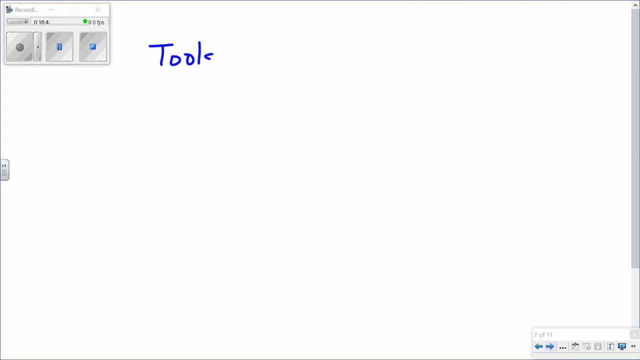 that you have so far for solving right triangles. If you know two sides, like we just did on that one, we're trying to find the hypotenuse or any of the sides. If you know two sides, what do you use? 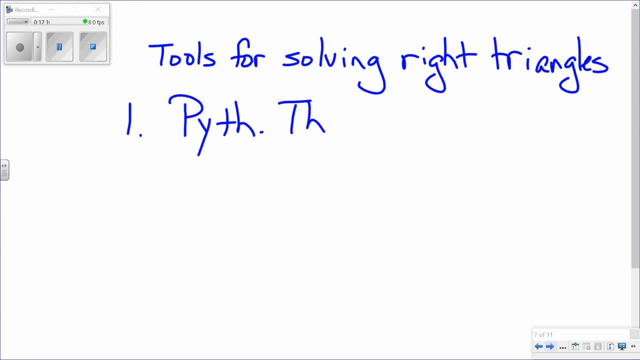 Pythagorean theorem. Pythagorean theorem: If you know, If you know two angles, what do you use to get the third Triangle sum? And then your other one is using your calculator with trig functions or inverse trig functions. But don't forget triangle sum and Pythagorean theorem. 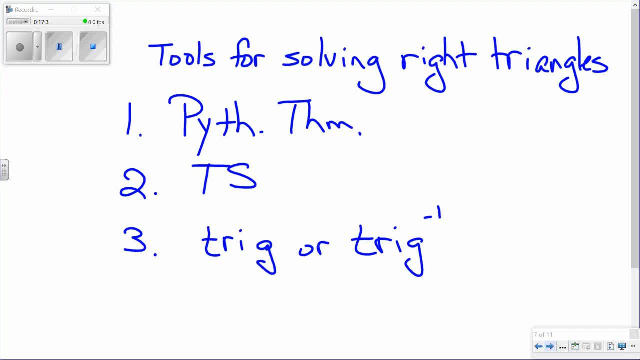 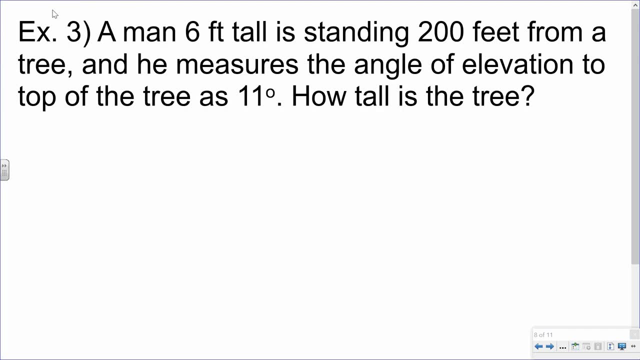 just because we're doing right, triangle trig, Okay, trying a word problem. now, With word problems, sketches are required. Please don't make them elaborate. I want you to still have time for your English homework, your social studies homework, whatever else you need to be working on. 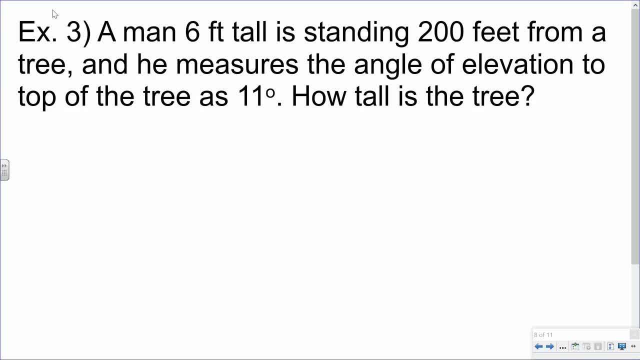 So you can either draw with just straight lines or very simple little sketches. It is fine to say: here is my tree Over here is my man who is six feet tall. He is 200 feet away. Now, technically, this problem is a man whose eyes are six feet above the ground. 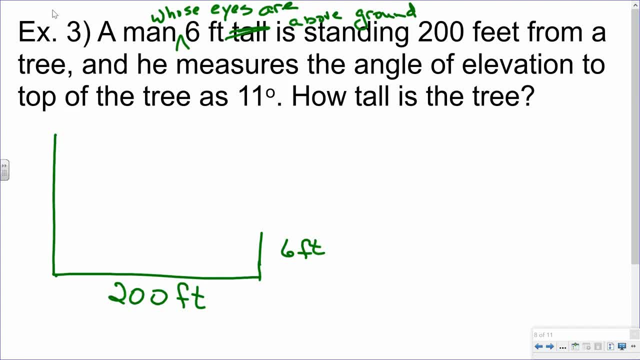 So I don't know he's really what. six foot four or something like that. If his eyes are six feet above the ground, He looks up at the top of the tree. Angle of elevation never has a vertical side, So I've got to draw my horizontal line in there. 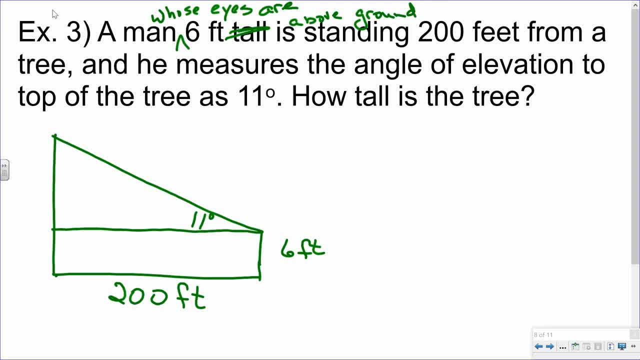 Eleven is right there, Horizontal line and the slanted line. That is his angle of elevation. How much does he tilt his eyes up? Is there a right triangle in this picture? So I'm going to call this side of the right triangle X. 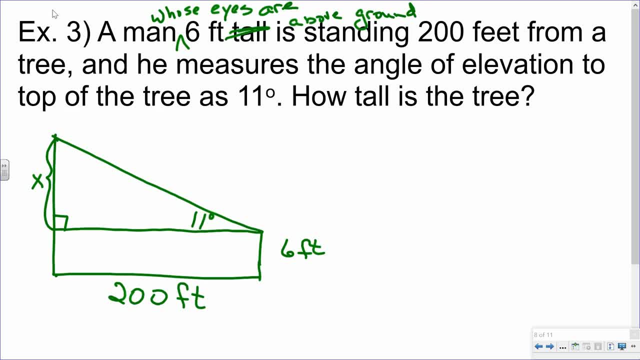 Who can tell me the ratio to set up to find X For 11 degrees? 200 is which side, X is which side? Which ratio do I need, Mia? can you help with that one? 200 is adjacent, opposite or hypotenuse. 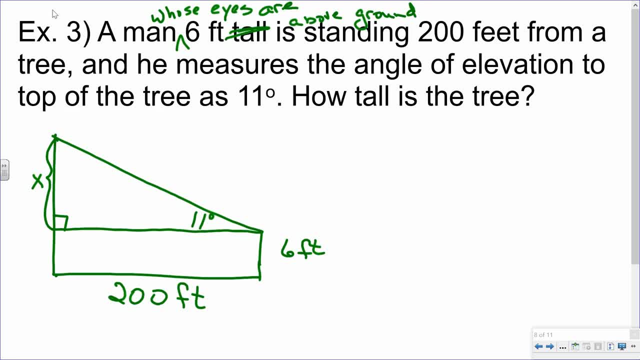 And X is if I'm using adjacent and opposite. which ratio do I need So I can say the tangent? The tangent of 11 degrees is X over 200. So X is 200, 10, 11.. I need your help with the calculator. 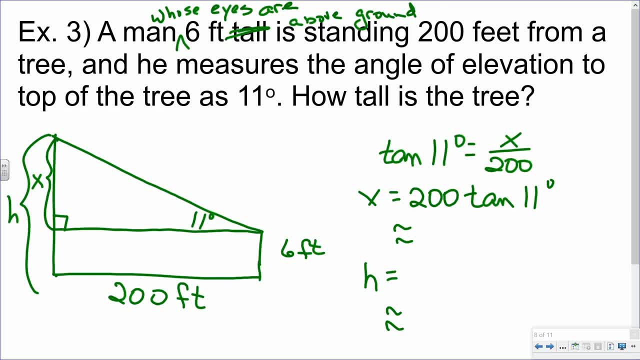 Raise your hand when you have a value for 200.. 10,, 11.. Sharon, you have one, So 38.876.. Anybody else get that? Thumbs up, thumbs down Is X. how tall the tree is. 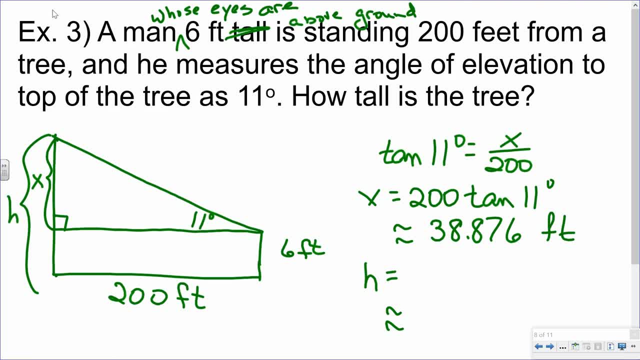 What do I have to do to get how tall the whole tree is? So the tree is 44.. 44.876 feet. So any questions with that? Now, if you want to do a little tiny bit of artwork, don't do anything more involved. 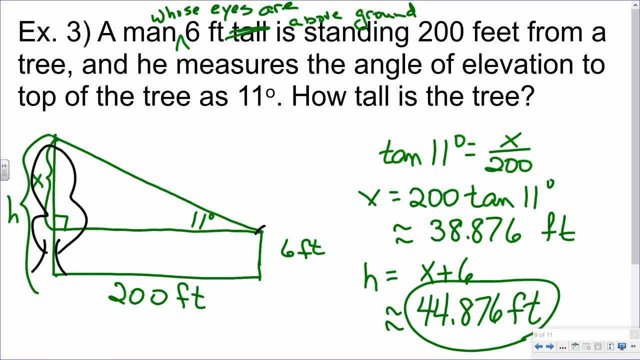 than something like that for your tree and something like a stick figure for your person. so it doesn't take real long. You can do that, or you can just do the straight lines Questions with that example. Okay, we're not going to do this entire problem. 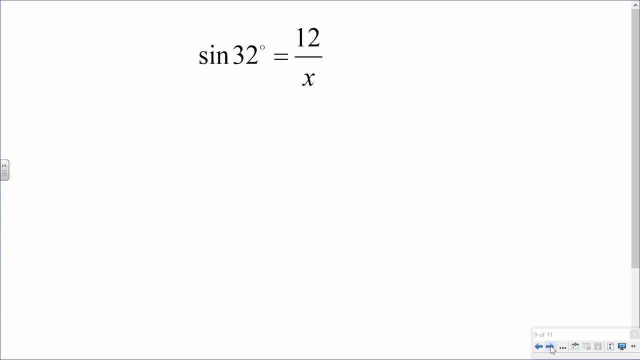 but sometimes when you set up the word problems, X is going to land in the denominator. when you set up your ratio, How do I isolate X when I see something like this: Will X be 12 times sine 32?, Holly, what do I need to do instead? 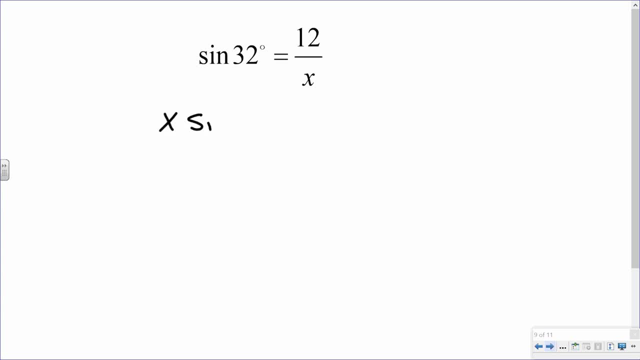 Okay, so if I multiply both sides by X, I have X sine 32 equals 12.. Then what? What would I do if I did 12 times sine 32?? Well, I would do the same thing. I'd do the same thing, but I'd do the same thing. 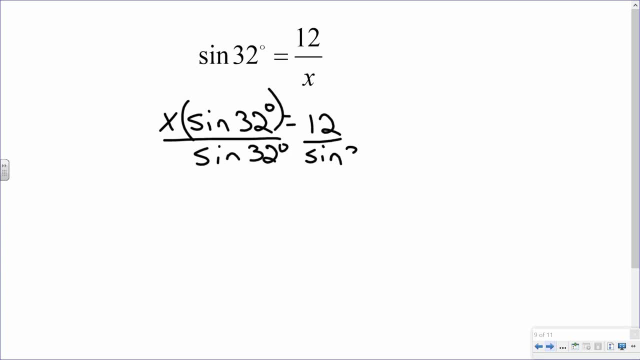 by dividing X by 32.. So to get X I really need 12 divided by the sine of 32 degrees. Now let me show you a shortcut that you may use for those Any you can put the sine 32 over one. 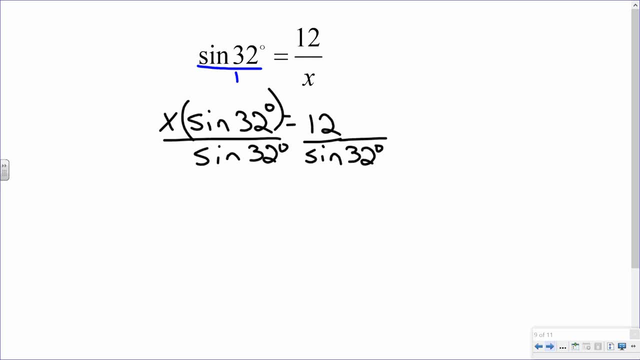 Any time you have a proportion, You may pick just one of the diagonals, It does not matter which one, and you may switch the two things on that one diagonal. So I'm going to put x up here on the left and sine 32 degrees over here on the right. 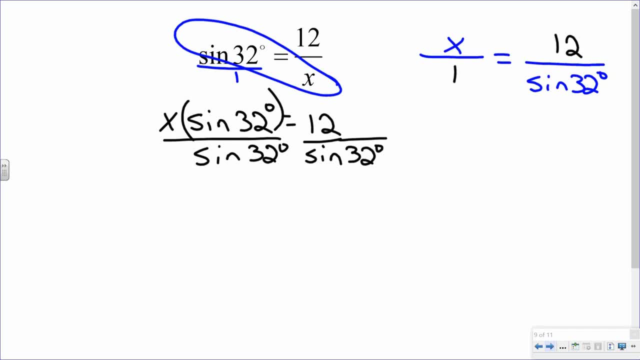 and you leave the other diagonal like it is. So that's another way to set it up to get that x is 12 over the sine of 32.. Okay, Numbers 14 and 15 on the worksheet that I'm giving you today are challenging. 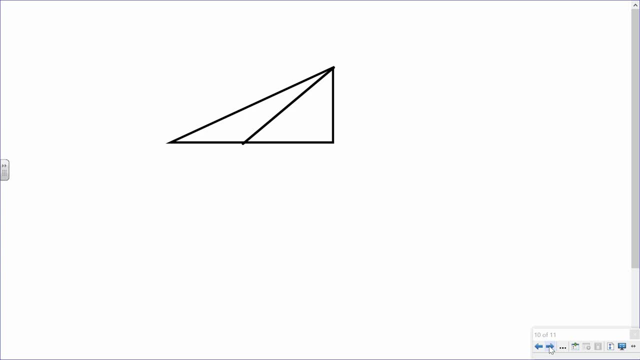 and they are problems kind of like this. We're not going to solve this one, but we're going to talk about the basic setup with it. So let's suppose we are out here somewhere and we measure an angle of elevation of 20 degrees. and we want to know how tall that thing is that we're looking at. And then let's suppose we move 50 feet closer and now the angle of elevation is 30 degrees. That is enough information. That is enough information to solve and find out how high that object is. 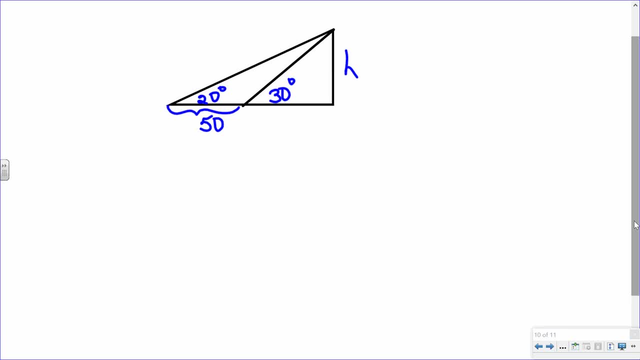 It doesn't look like it at first. Now, if I were to start out with this triangle on the right, I could say that the tangent of 30 degrees is opposite over adjacent, so I probably need to label that side with something That means h is x 1030 degrees. 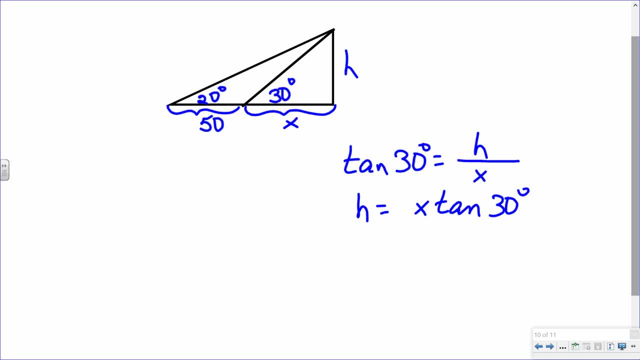 Okay, then if I am over here I can say that the tangent of 20 degrees is also opposite over adjacent. but now my adjacent side of the right triangle, not the obtuse triangle, is 50 plus x. So basically I've got a system with h and x. 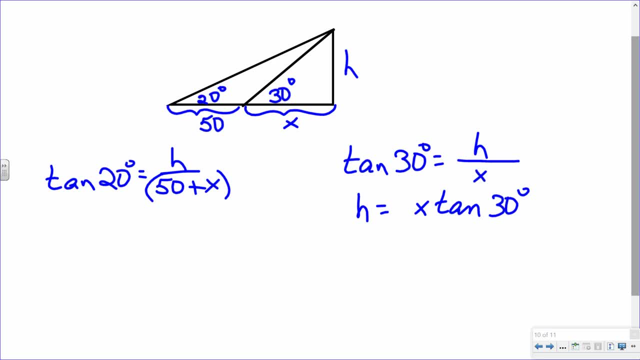 two equations with h and x in there. So for this one I can say that h is the tangent of 20 degrees times 50 plus x. Those are both h, So I can do substitution and I can say that the tangent of 20 times. 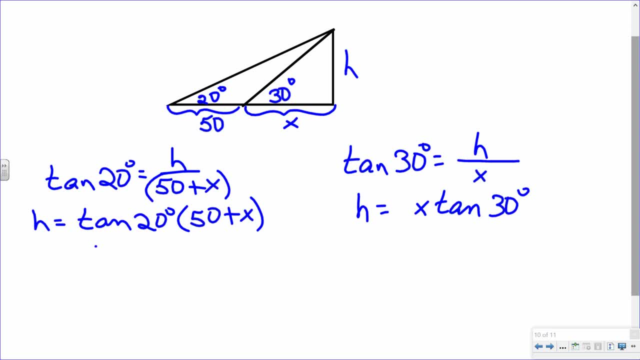 the parentheses. 50 plus x is x times the tangent of 30 degrees. If I distribute, I have 50 tan. 20 plus x. tan 20 is x 1030.. Can I get both x's on one side? Can I get both x's on one side? 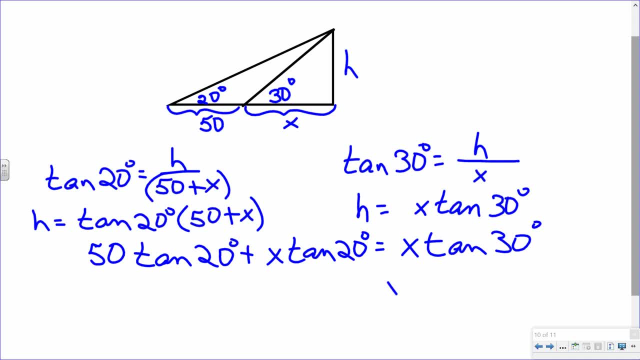 Can I get both x's on one side? Factor out the x And then if I divide by my long parentheses will I have x. Then if I want h, I can take whatever that is times the tangent of 30 to get there. 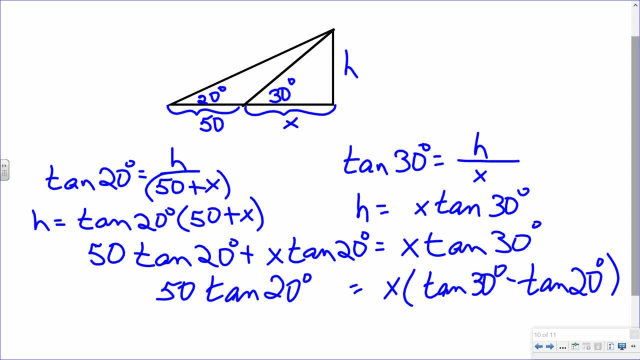 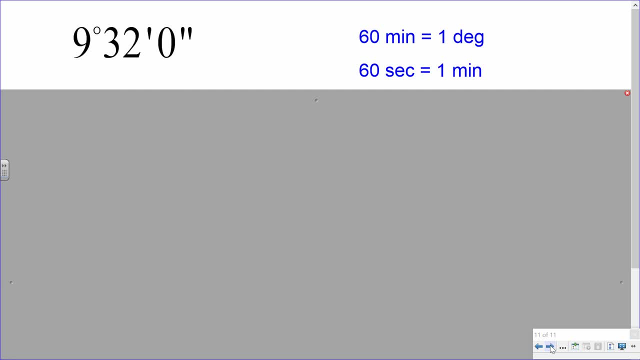 So you get that strategy. You'll need that on 14 and 15.. Okay, final thing I want to show you today. Sometimes problems talk about fractions of degrees. Each degree has 60 minutes and, just like time, each minute has 60 seconds. 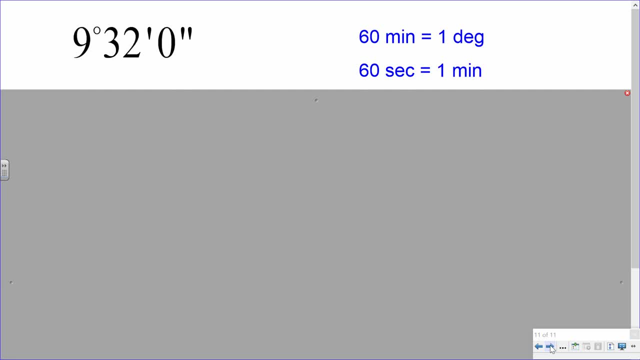 So this is 9 degrees 32 minutes 0 seconds. I'm not going to be mean enough to give you one that really has seconds in there, But I might give you 9 degrees 32 minutes, And that means